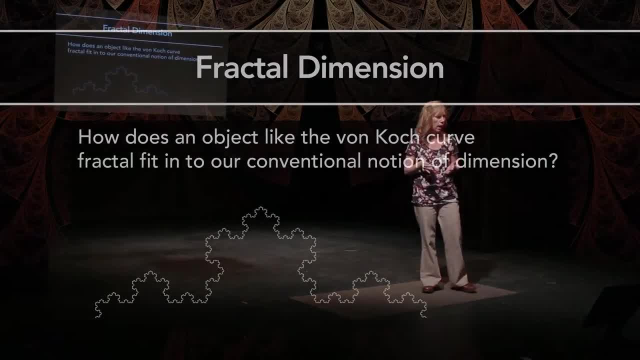 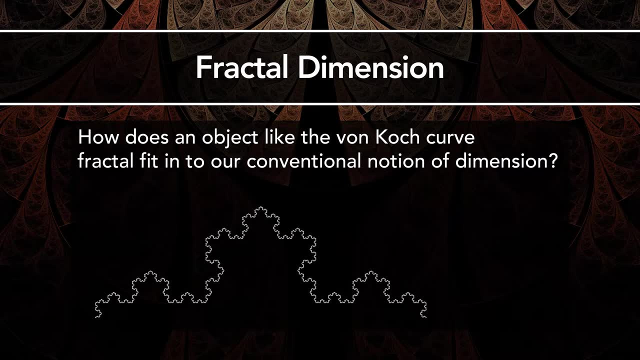 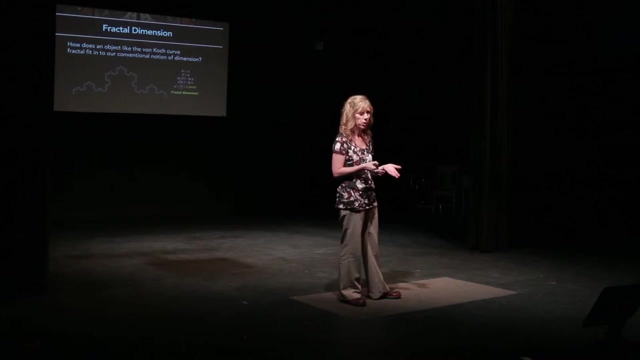 fractals. And so if we apply this formula to an object like the Van Gogh curve, a fairly simple looking fractal, we see that the dimension is approximately 1.26185.. Fractal dimension: Fractals live between dimensions. What does this mean? Well, the Van Gogh curve pictured here, 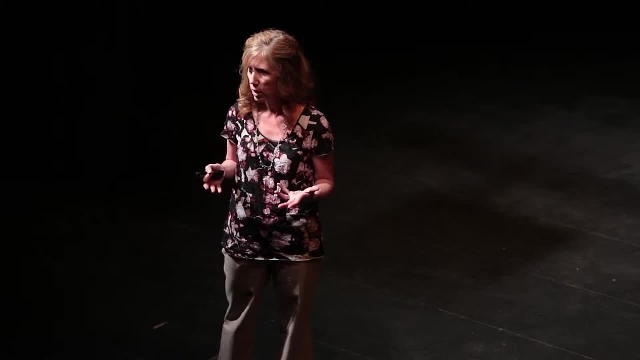 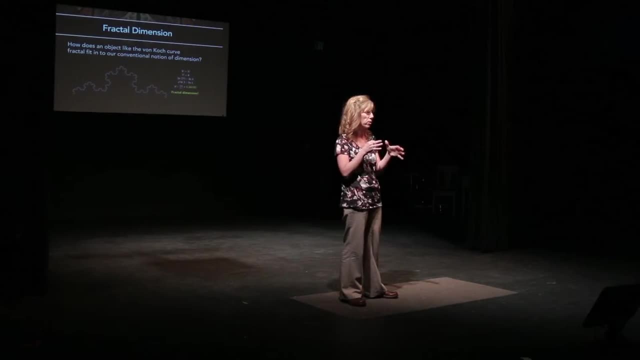 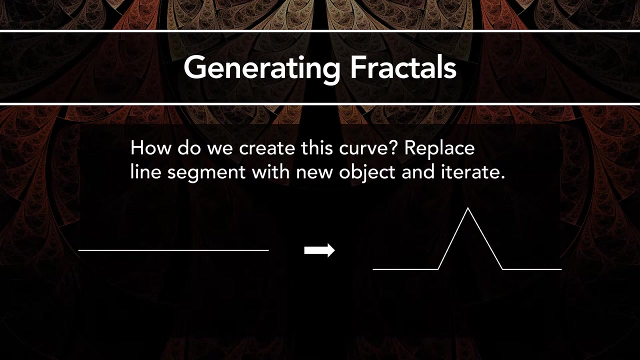 has some characteristics of one-dimensions. It's generated using line segments which are one-dimensional, but it doesn't live in the bounds of one dimension. It's sort of infinitely edgy and that pushes it Right outside the one dimension. So how do we generate fractals? Well, fractals are the result. 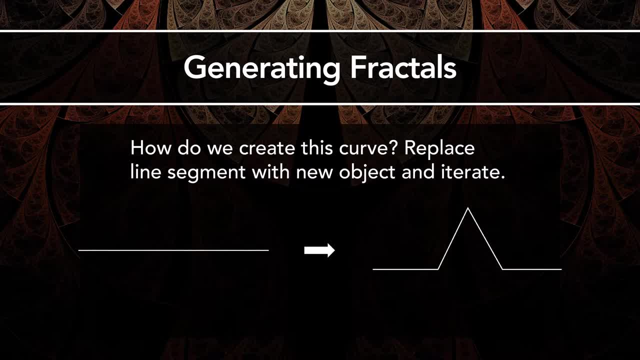 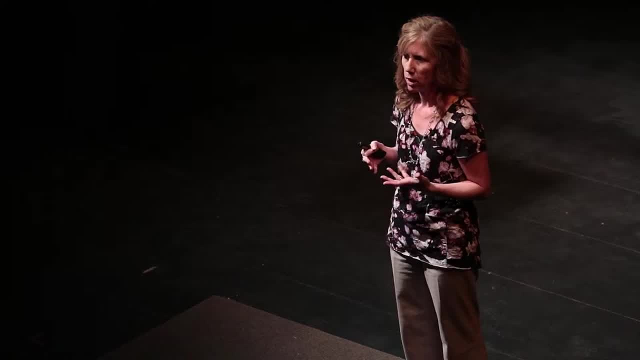 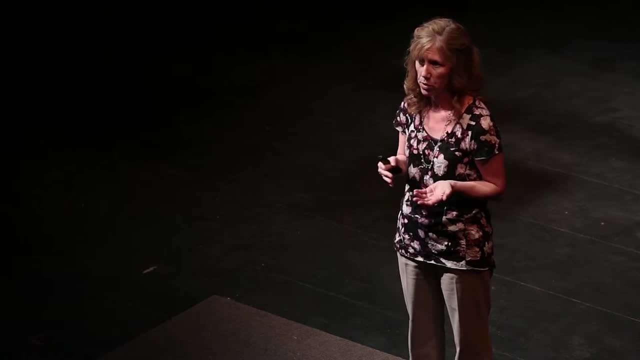 of an iterative process that's repeated infinitely many times, And so, for the Van Gogh curve, there's a geometric way to view this, And so, starting with the line segment that you see pictured here, we're going to replace it with the object, and we'll call this new object the 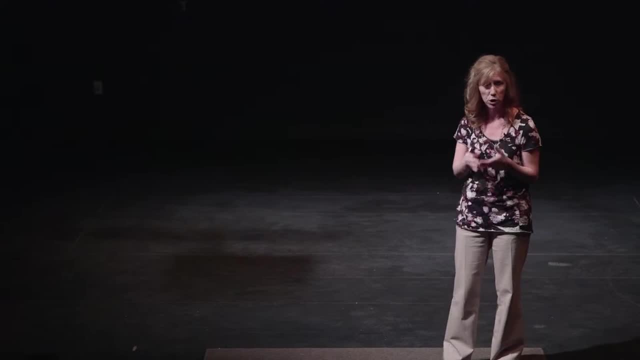 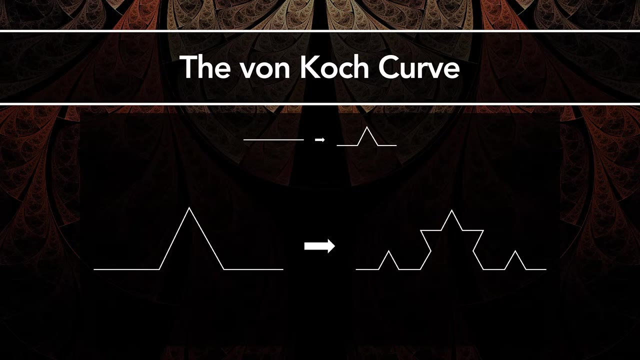 first iteration. We then take that first iteration and we're going to take the first iteration, which is made up of four line segments, and we replace each of those line segments with that object, again, generating the second iteration. And we repeat again and again until after. 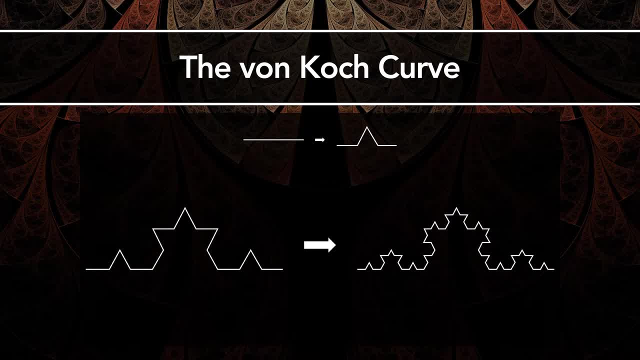 infinitely many repetitions, we generate the Van Gogh fractal. This fractal that you see pictured here maybe looks somewhat natural, maybe almost like a coastline. Well, except, it seems a little bit too regular. So what if we throw a little bit of the fractal in the middle of the line segment? 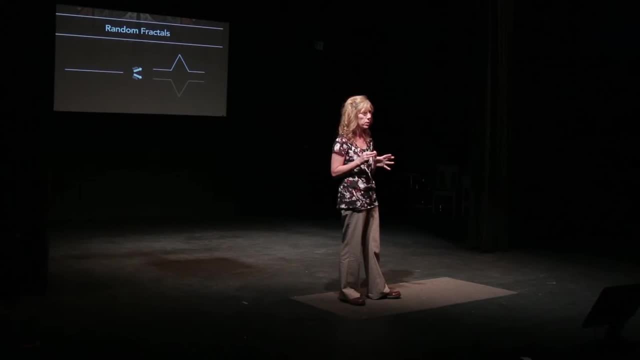 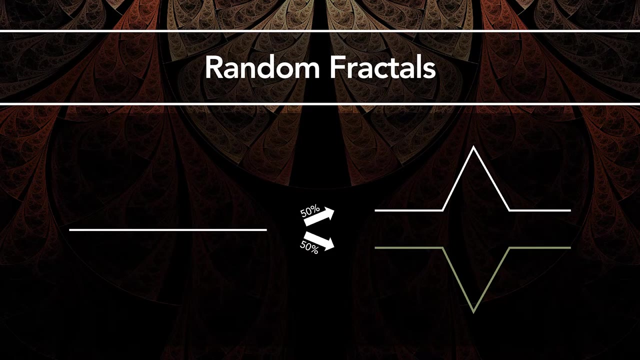 a little randomness into this. So 50% of the time we'll replace our line segment with the object that we started with. The other half of the time, we'll replace the object, the line segment, with the object that you see below the green with the triangle pointed down. When we do this, 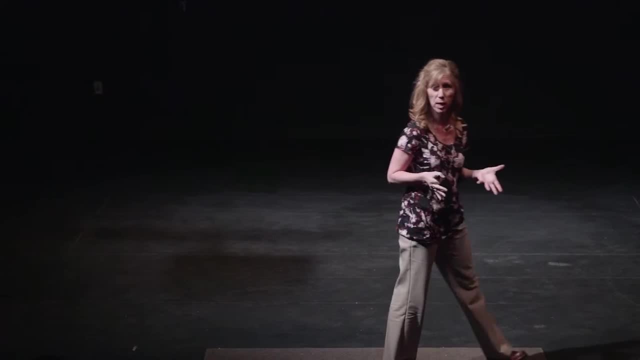 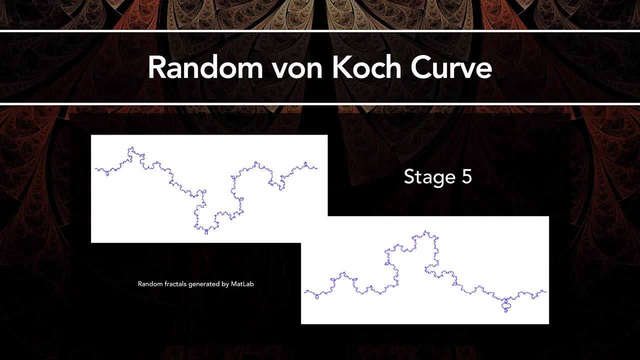 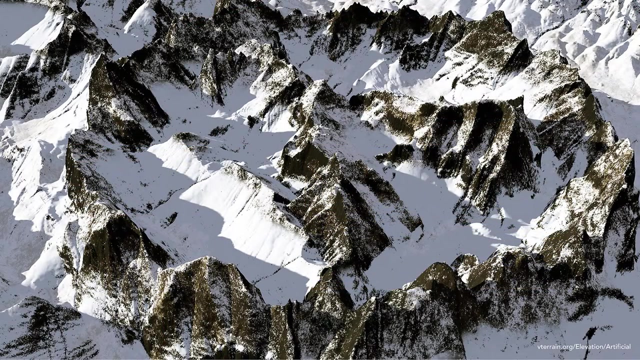 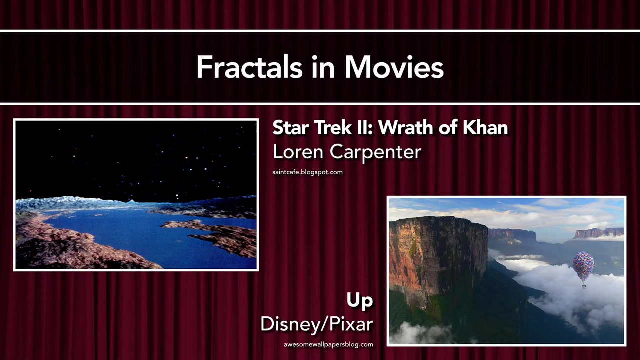 the fractal that's generated much more closely resembles a real coastline. Random fractal generators are being used to construct landscapes like the ones you see here. They're almost indistinguishable from photographs, but these are computer-generated fractal landscapes, And this technology is being used to create landscapes and animation in movies.